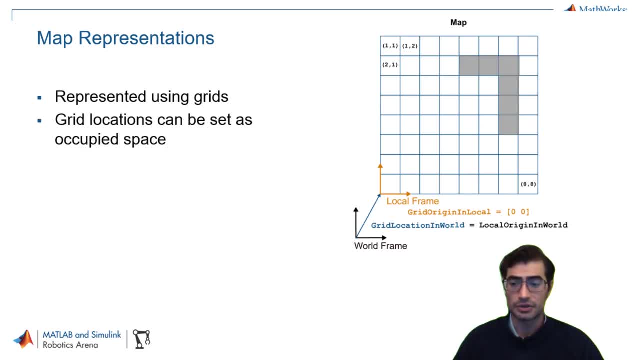 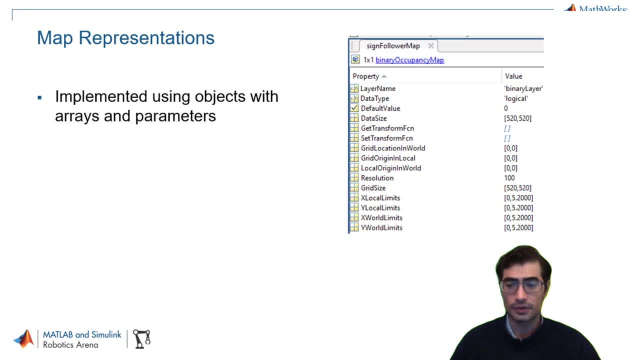 generally represented using grids, where the grid positions or locations can be set as either free or occupied space. In turn, this grid information is implemented in software using objects that will contain or encapsulate these different arrays and parameters. The object will contain information such as the grid itself, the map limits, the 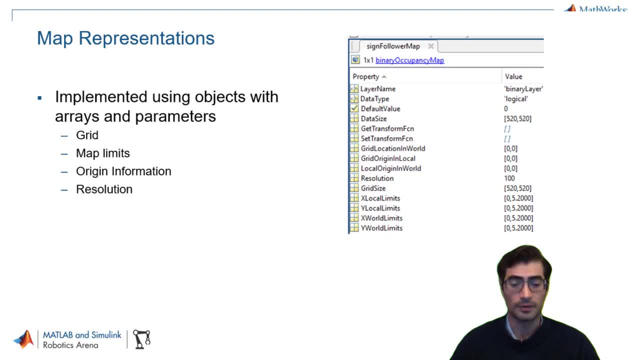 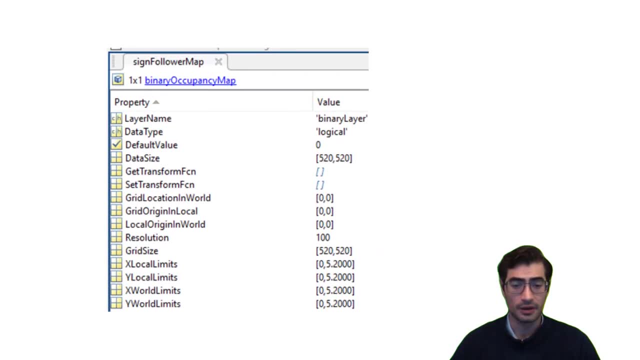 information of the origin and also the resolution of the map itself, so that it can be correlated to the physical world. In this case, we can see the parameters contained within a Matlab mapping object called the binary occupancy map, And here you can see that you have access to your X and Y local limits- X and Y world. 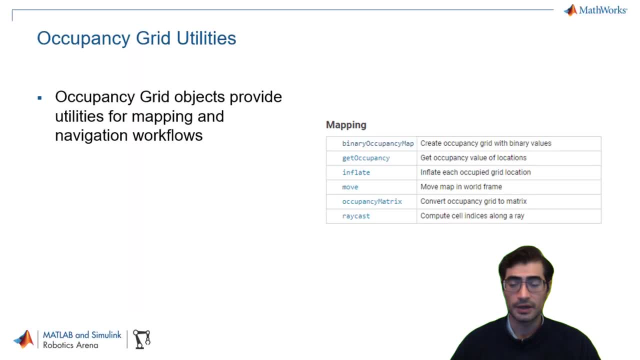 limits and a whole other array of information. Having a map defined as an occupancy grid will give you access to important utilities. These utilities will help with your robotics workflow, especially navigation workflows, by letting you access the information in the map, like getting the occupancy or inflating. 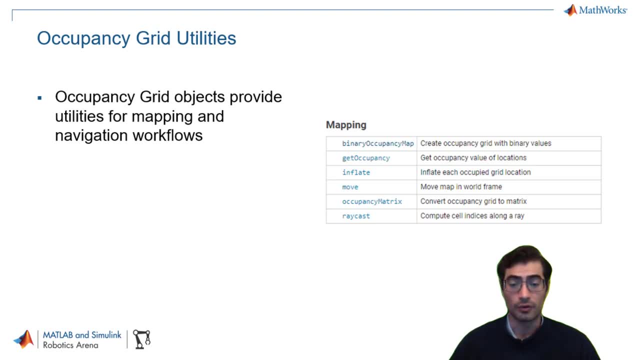 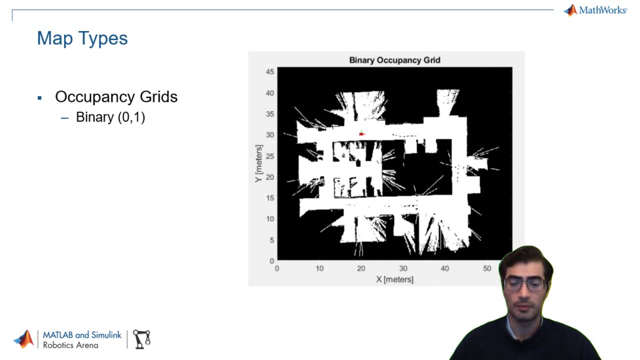 the occupied spaces in the map to prevent the robot from running into obstacles or even moving certain portions of your map to account for different coordinate transformation that your algorithm might require. Maps can come in several different types. Occupancy grids, in particular, can come in binary form, which will only specify whether 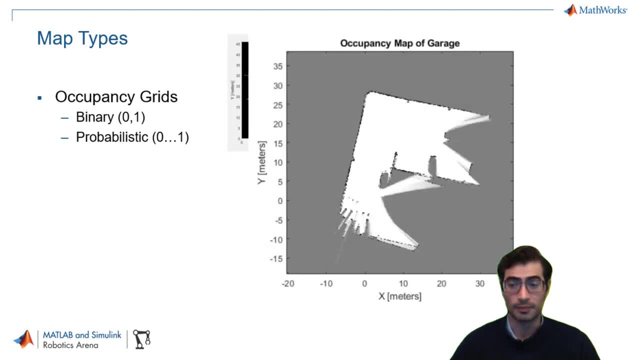 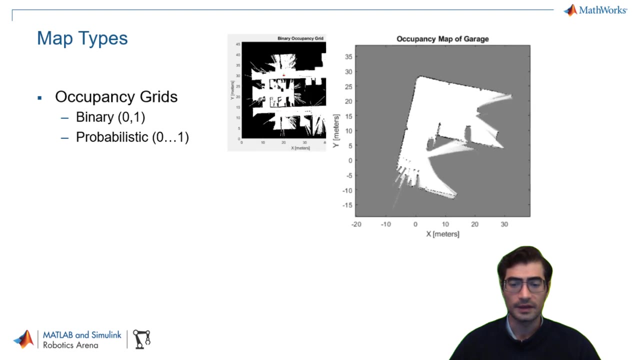 a space is free or occupied. They can also be probabilistic occupancy grids, which will give you a more granular set of information, ranging from, let's say, 0 to 1, that will give you the probability of a certain section or portion of the grid of being occupied or not. 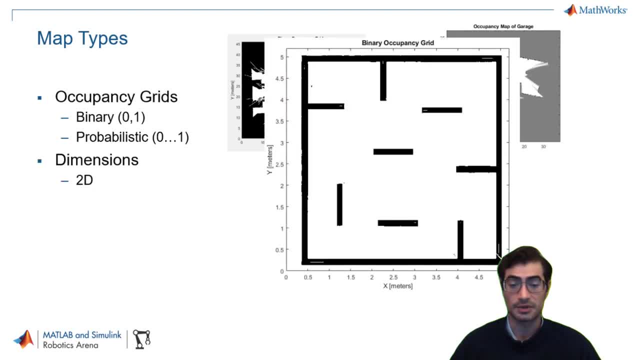 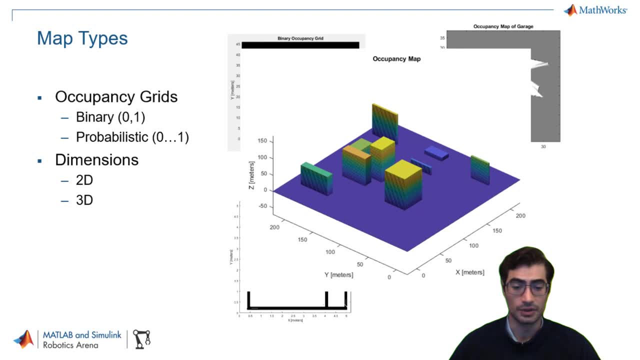 And then, finally, they can be split up by dimensions. Occupancy maps can represent spaces in either two dimensions or three dimensions, Depending on the application that you're going to be using these maps for. With the brief introduction on mapping for robotics and autonomous systems application. 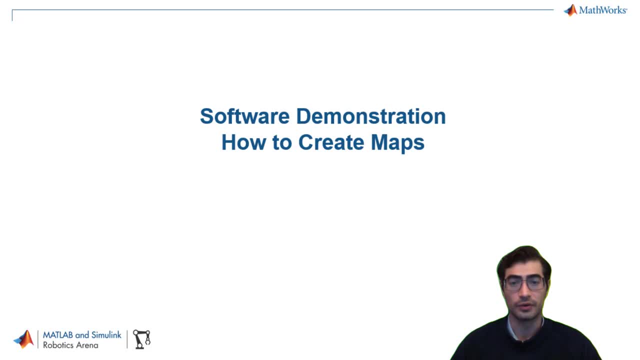 we will now move over to a hands-on software demo to show you how to create maps. If you'd like to follow along or are interested in the files we will be using here, you can find the link to the files in the description below. 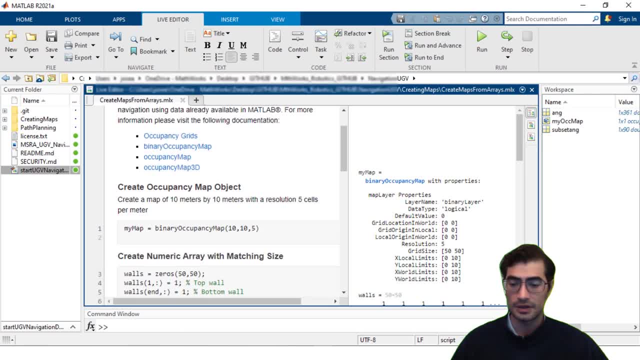 This example live script will show you how to create maps from arrays. In this case, we are creating a map to correspond to an environment that is 10 meters by 10 meters, And we are trying to create it with a resolution of 5 cells per meter. 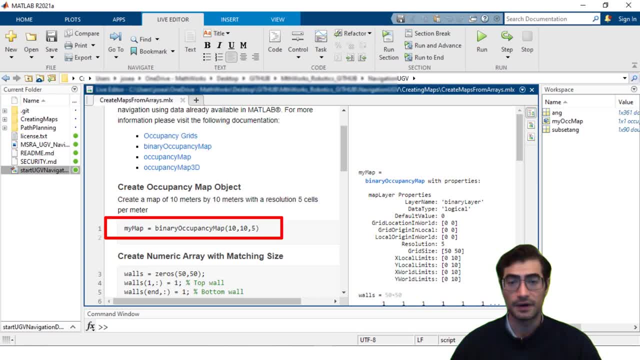 For that we used the binary occupancy map method and then specified the dimension or resolution of our map. You can see on the right in the live script that we now have a map that's of binary occupancy map type with the following properties, Some of which are the grid size which corresponds. 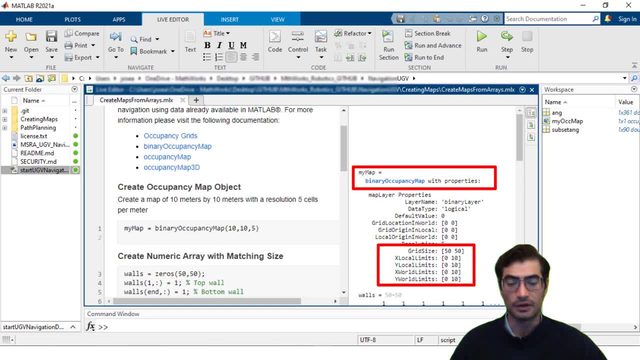 to our dimensions, times, the resolution and then different local and world limits that we have set for it. Then we would create an array that we Carries in the binary customstatables table to express how the blob check the visibility on the map and새 rate that we've set for it. Then we would create an array that 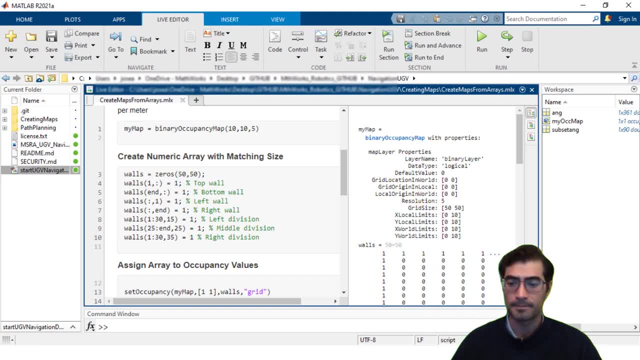 can use for setting the occupied space within the map. In this case, we're creating a variable called walls, that is, of 50 by 50, which corresponds to the grid size of our map, and then setting the occupied space on the relevant locations, in this case for the walls and some divisions, by using the value. 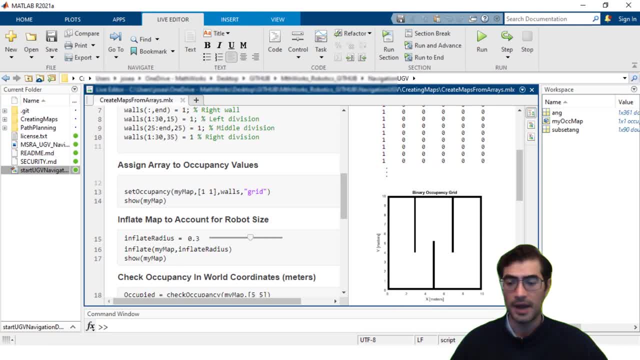 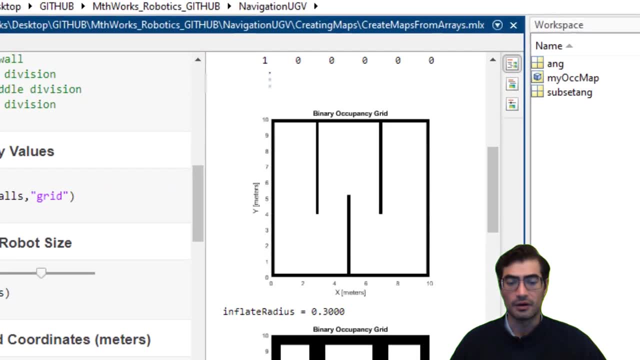 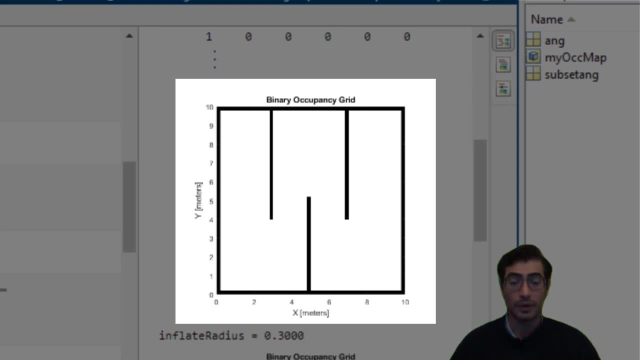 of one. Then we update the map that we've created, called my map, by using the method set occupancy and passing the variable we created, and this is what our binary occupancy grid will look like. once we've assigned the occupied space using the array, We can see in the visual that the walls 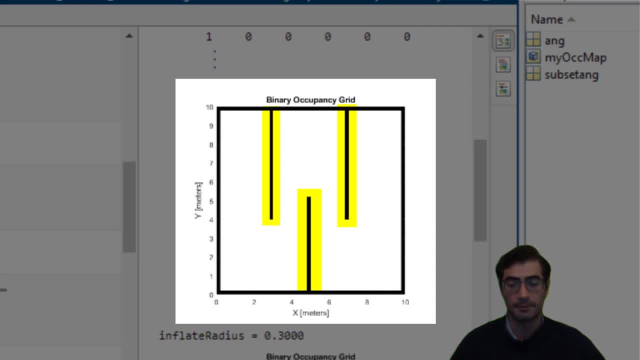 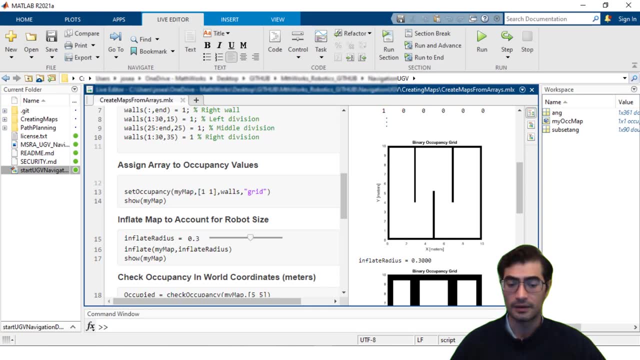 are now corresponding to occupied space and we have three divisions in the middle of the map. Now one of the utilities that occupancy grids will provide you is the ability to inflate your occupancy map. Inflating your map means that you can have a safety factor for your robot radius. 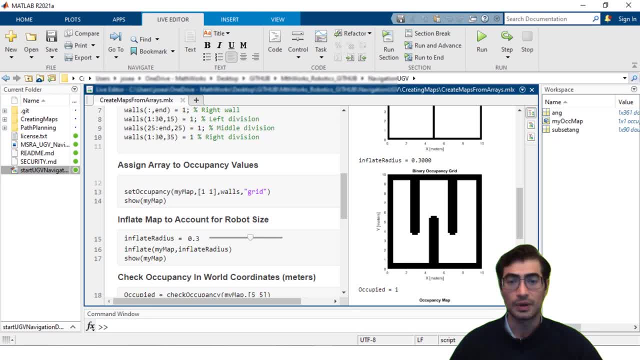 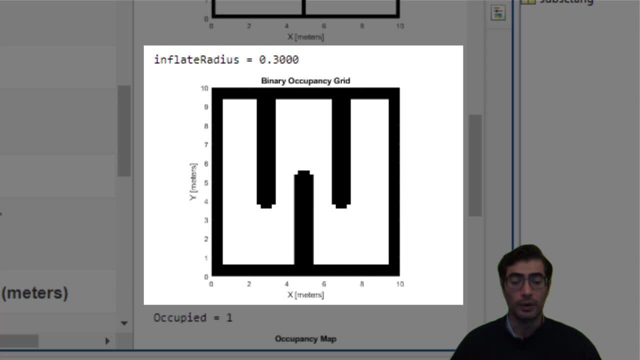 so that it won't run into the occupied space. In this case, we can set an inflate radius of 0.3 and then use the inflate method to update my map. You can see that we will not have much thicker walls, which will then translate into a bigger safety factor when using 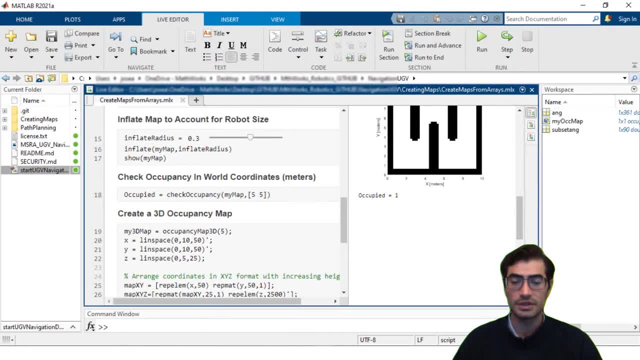 any motion or path planning algorithms. If you're interested in individually checking whether a portion of that map is occupied, you can always use the method check occupancy and pass on your map and then the location that you would like to check, and in this case we can. 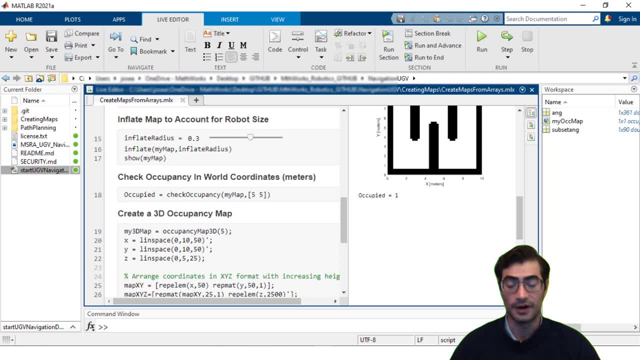 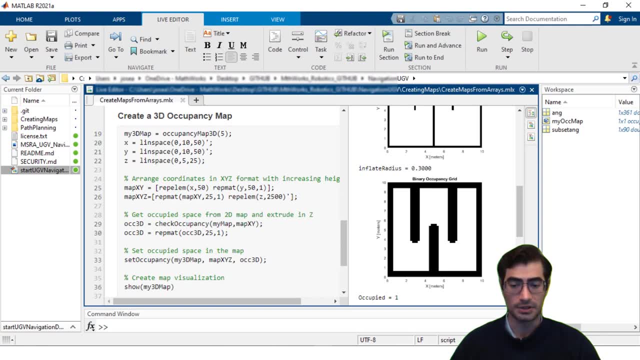 see that if we want to check whether the location corresponding to positive 5 meters and 5 meters is occupied, then we get the answer is true. You can also create 3d occupancy maps. In this case, I'm creating a placeholder array to store the map information and then I am extruding the current. 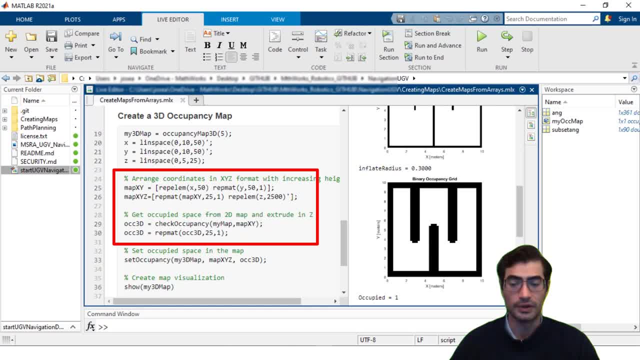 map that I already have in two dimensions. by adding a z coordinate to all of the elements, I will set the occupancy using the set occupancy method by passing my coordinates array and my occupancy array, and you can see here how we now have a three-dimensional version. that has been 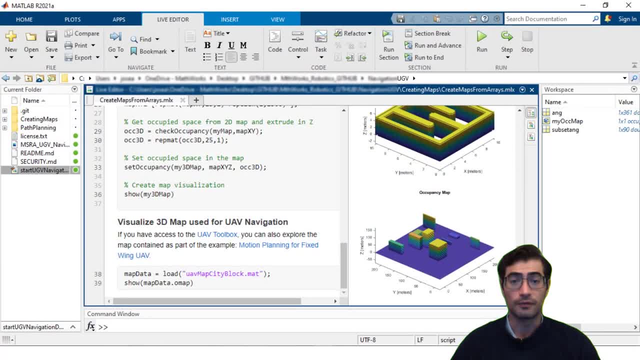 extruded on a z dimension. 3d occupancy maps are also very popular for UAV applications, so if you're interested in mapping for UAV navigation, we recommend that you take a look at the documentation for the MATLAB UAV toolbox. However, creating these maps by specifically, 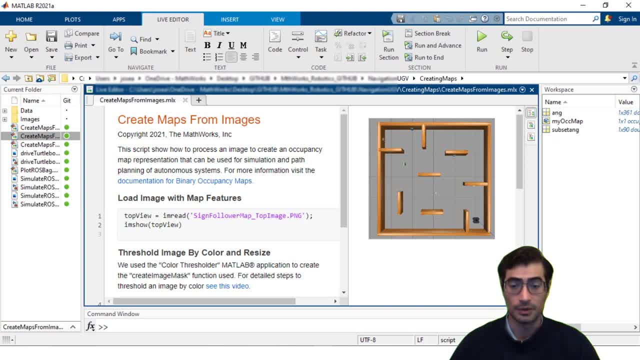 defining each of the individual grid locations using arrays can be very time consuming. A much more efficient way of creating maps is by processing images of your current environment and then using those to set the occupied space in your maps. One way to do this is by thresholding an image by its color. In this example, we have a top view image of our 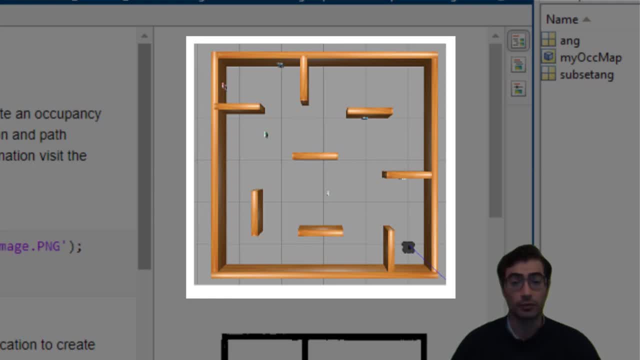 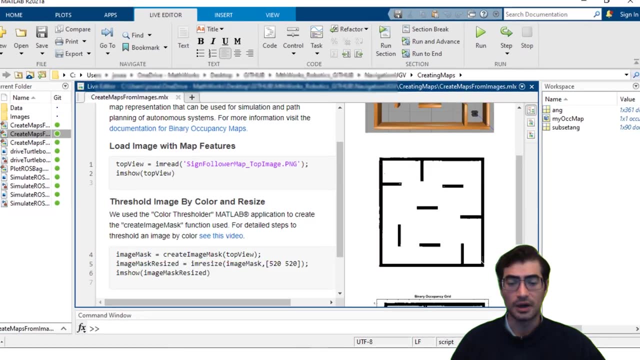 TurtleBot 3 map that contains all the relevant walls that we would like to prevent our robots from running into. So we would load that image into MATLAB and then threshold it by color. You now have a black and white version of the map that contains only the information from the walls. 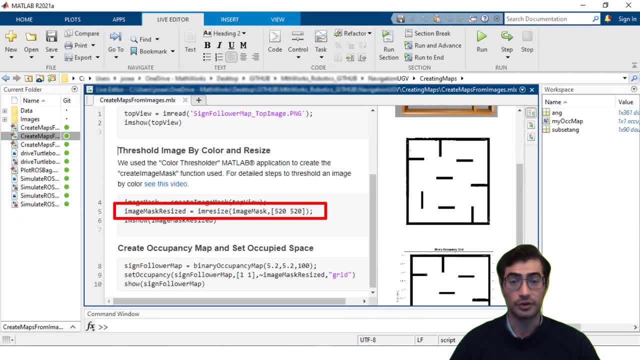 In this case, we will resize it to a resolution of 520 by 520 pixels, since we're trying to create a binary occupancy map with length and width of 5.2 meters and a resolution of 100 cells per meter. After we set the occupancy in our object, we can see the finalized version of our binary occupancy grid. 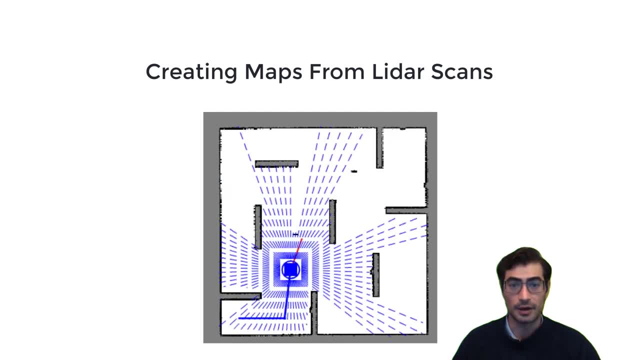 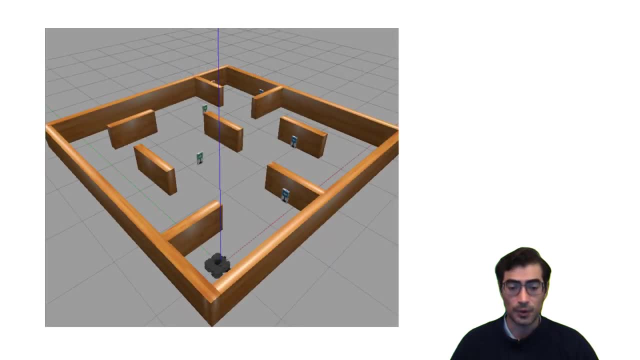 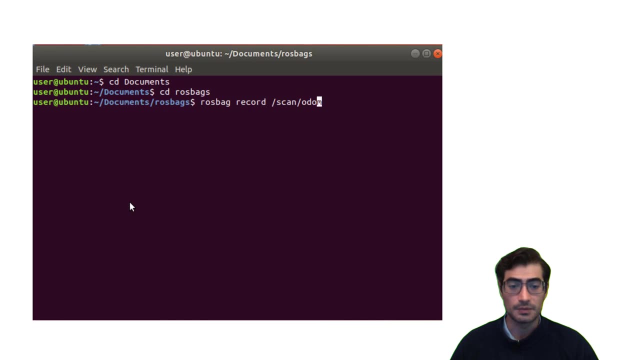 To create maps of your robot environments would be to use laser scanners to capture information from the different surfaces. In this case, we're using a simulated robot that is ROS enabled and we are using the ROSback functionality in order to record the laser scans at each point. 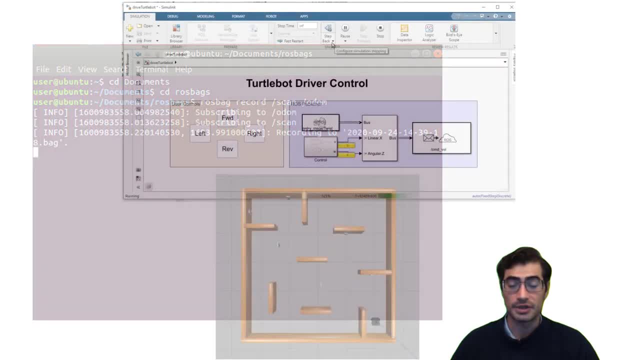 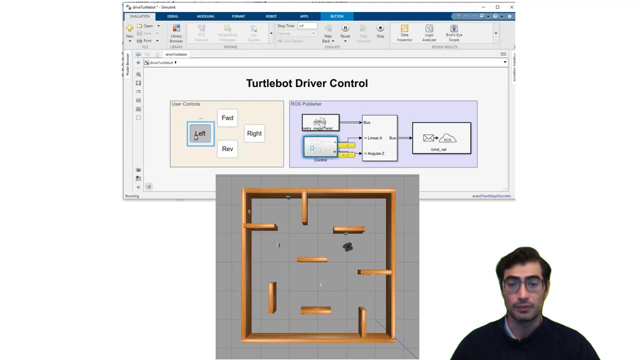 in time and the odometry of the robot. For the purposes of our demo, we're using a Simulink model that controls our robot so that we can drive it around the different paths within the environment and capture data from all the relevant surfaces, or walls, in this case. 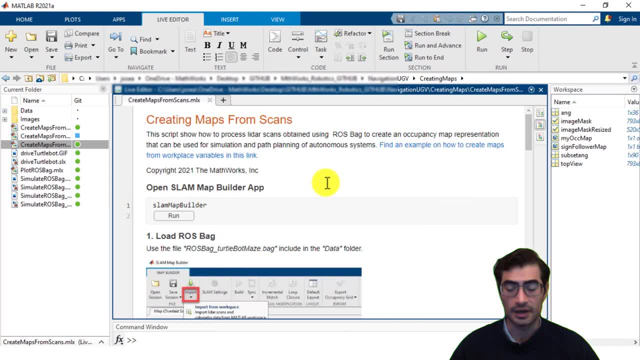 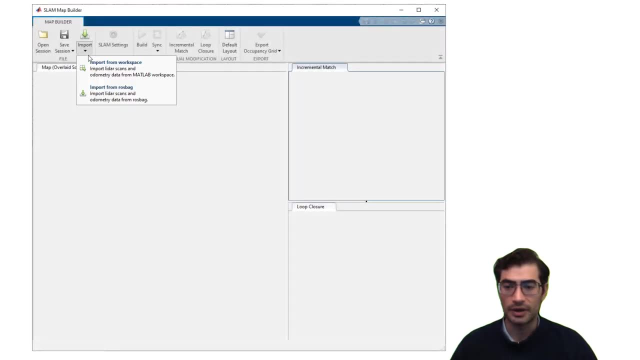 Once we have a ROSback containing the odometry data and the lighter scan data for the exploratory run we just performed with our robot, we can then go to the MATLAB app menu and select the SLAM map builder app. In the SLAM map builder application, you can import your ROSback file. 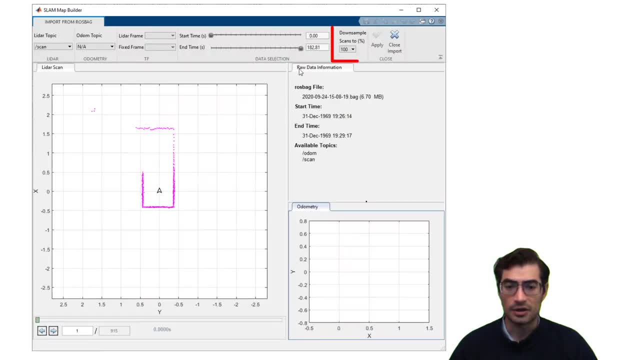 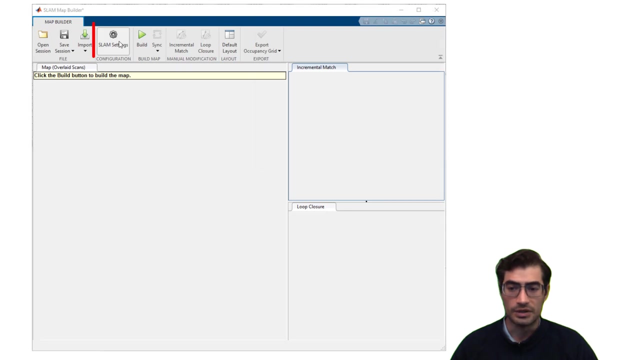 and select a downsampling scale for your scan so that the algorithm can run more efficiently and take less time. In this case, we will downsample to 50 percent of our scans and apply those changes. Then we will adjust our SLAM settings. In this case, we will change our optimization interval. 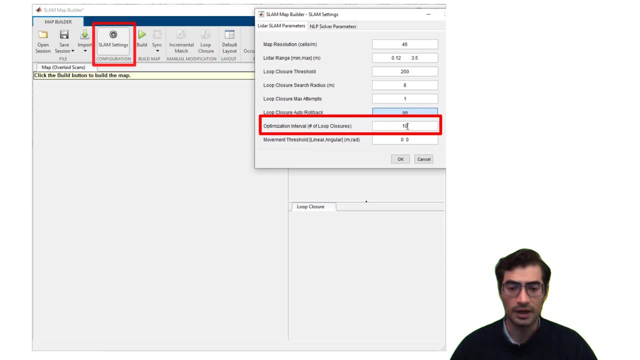 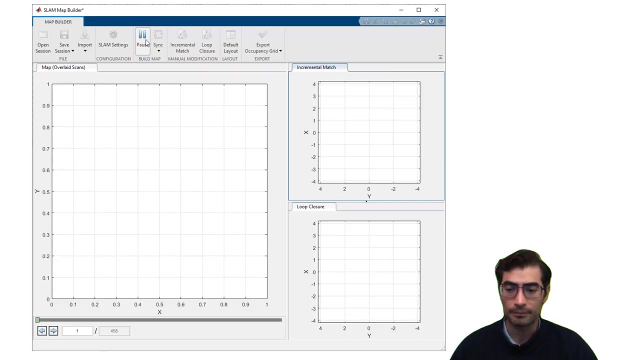 to 10 loop closures. If you want more information regarding the SLAM settings, you can check the documentation links in the example. And finally, we can click the build button on the app. The application will start processing all the different scans and building one map from all of. 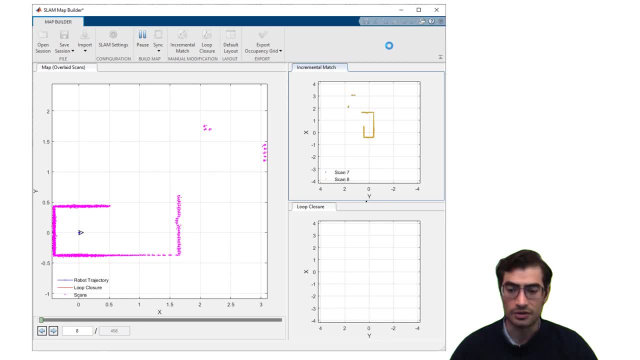 them. In this case, you can see how the application is surfing through the scans using the progress bar and you can see how the map gets more information added to it with each new scan that is correlated into the algorithm. In this case, we will fast forward to. 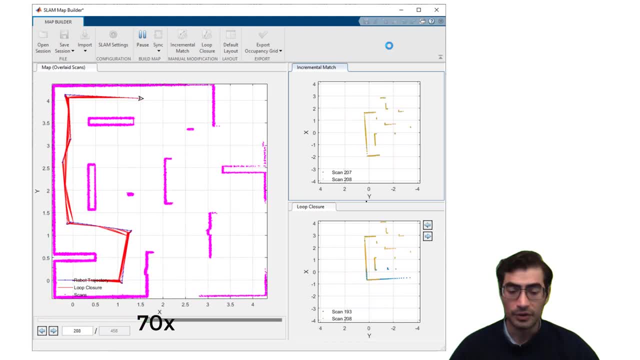 the end of the map building process to show you the end result. But you can adjust your SLAM settings in order to make this process go faster or slower, depending on the accuracy you need and the data that you have. Finally, you can export your occupancy map directly from the SLAM map. 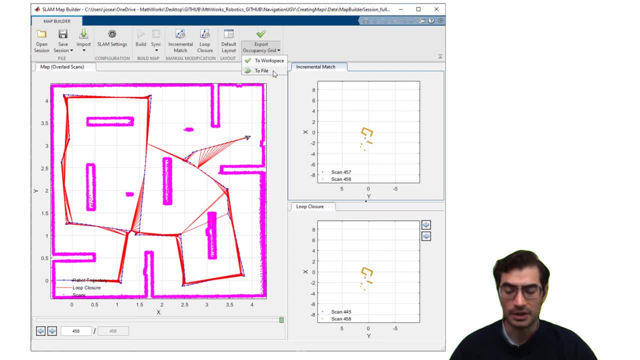 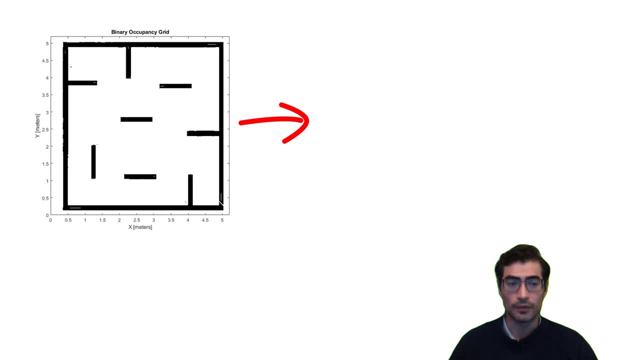 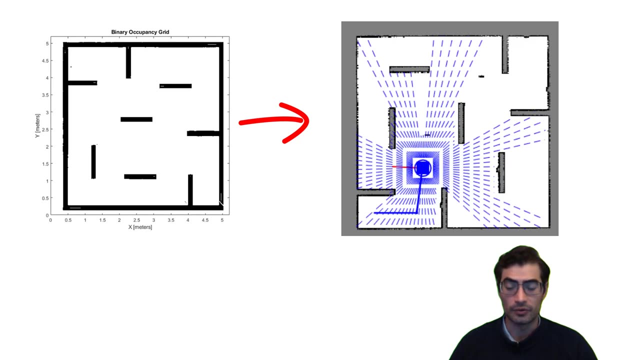 builder app and you will end up with the mat file containing the occupancy map that you can use for other workflows. Now that you have the digital representation of your robot environment, you can use it for either motion planning or path planning. You can use it for prototyping and simulation of your robot or autonomous system. 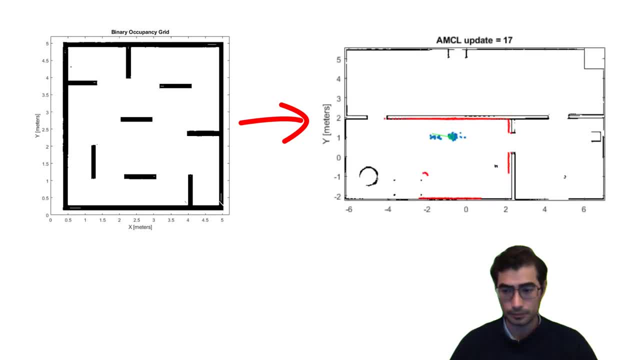 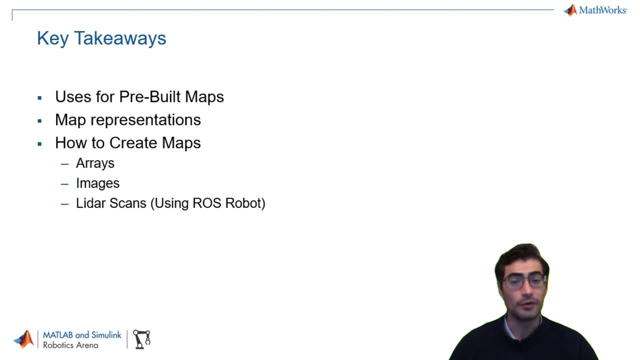 or other algorithms such as monte carlo localization. In this video, we covered the different uses for pre-built maps for robotics and autonomous systems, the different map representations and how to create these maps from either arrays, images or lidar scans that can come from your ROS enabled robots. 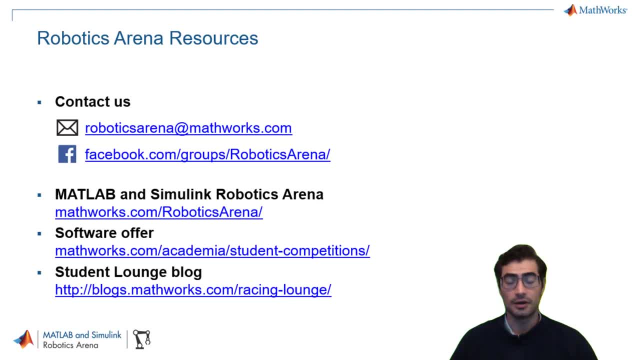 If you have any questions, feel free to reach out to us at roboticsarenacom, or feel free to check out any more of our videos and resources available on our website. Thanks for watching.